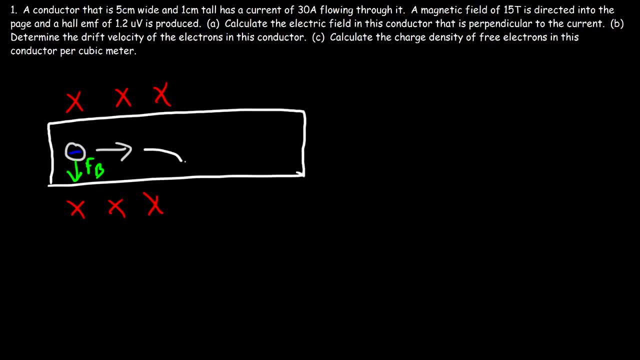 downward direction, and so it's going to travel in that direction. So what's going to happen over time is that there's going to be a buildup of negative charge at the bottom, and because the top part is electron deficient, it's going to have a positive charge, And so there's going to be a voltage across the conductor. 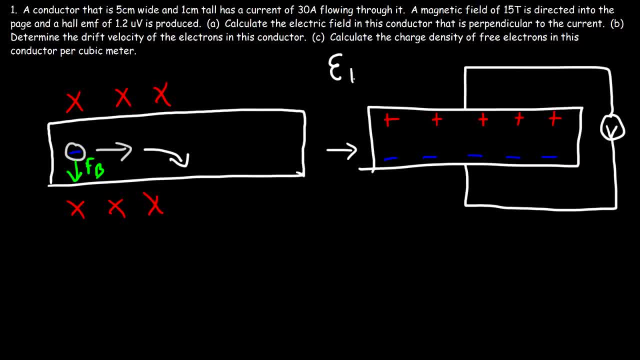 That voltage is known as the Hall EMF. So electrons will flow from this side and back to the other side, And so there's going to be a small voltage across that conductor. Now there's also an electric field that emanates from the positive 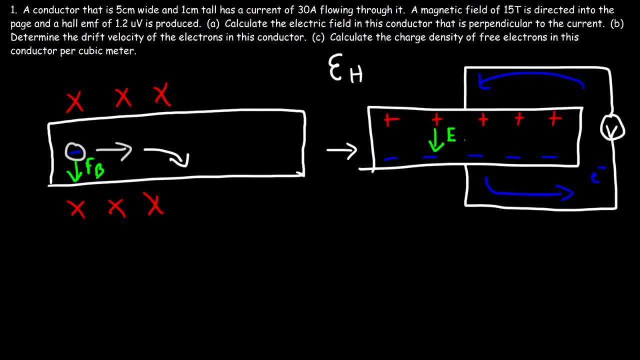 charge and flows towards the negative charge, And in part we need to calculate that electric field in the conductor, which is parallel to the current. So if the electrons are moving towards the right, conventional current is flowing towards the left, that is, in this direction. Electric field is equal to the. 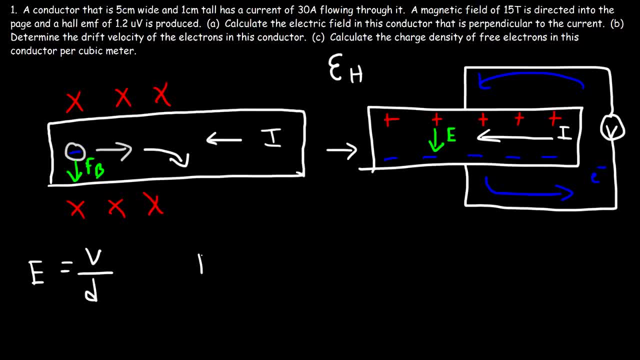 voltage divided by the distance. So in this case the voltage is the Hall EMF and the distance is the width of the conductor. So it's going to be 1.2 microvolts, or 1.2 times 10 to the minus 6.. 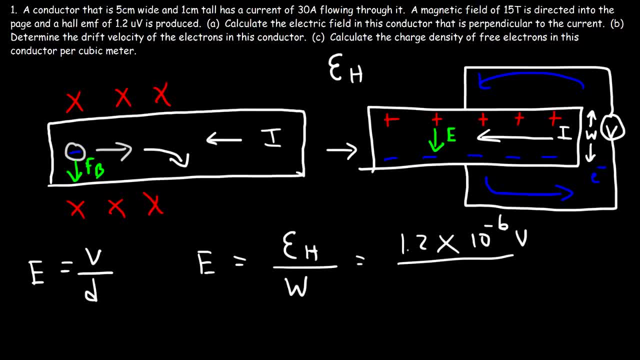 volts divided by the width, which is 5 centimeters wide, or 0.05 meters if you divide it by 100.. So the electric field in this example is 2.4 times 10 to the negative 5 volts per meter. So that's the answer for Part A. Now let's move on to 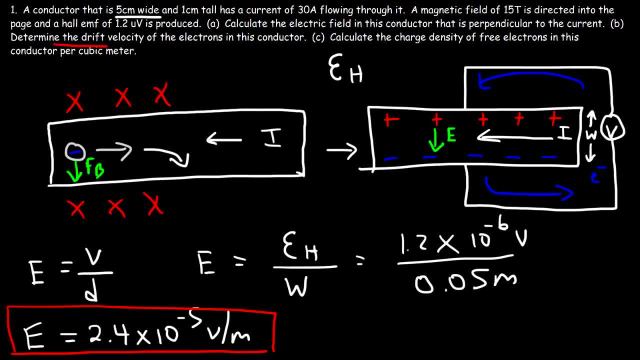 Part B, Determine the drift velocity of the electrons in this conductor. So how can we do that? So let's focus on the electron. We have an electric field that is going in a negative y-direction. A proton will flow, a force that will accelerate it in the 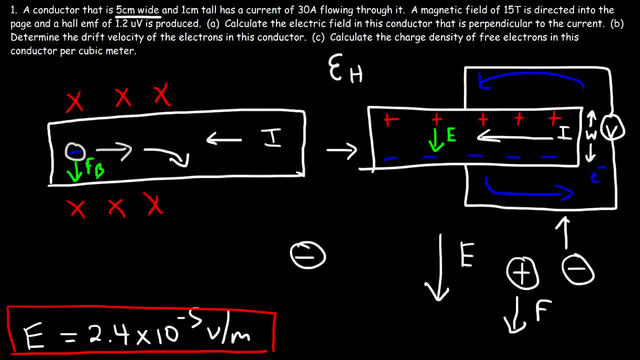 direction of the electric field, A negative charge will flow, a force that will accelerate it opposite to the direction of the electric field. So because the electric field is going in a negative y-direction, the electric force exerted on the electron is in the positive y-direction and the magnetic force is in the 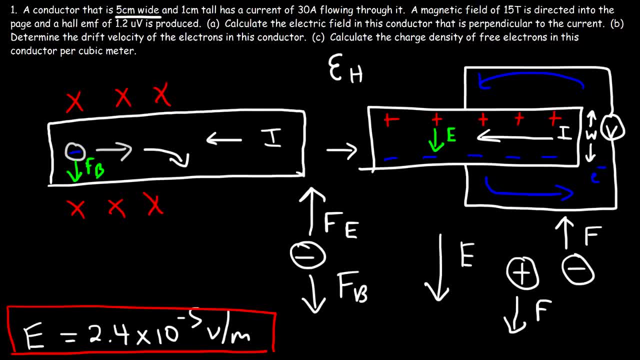 negative y-direction. Now, when these two forces are the same, the EMF generated will be in a state of equilibrium. So what we need to do is set those two forces equal to each other. So let's talk about this. As the electrons travel in this direction, we 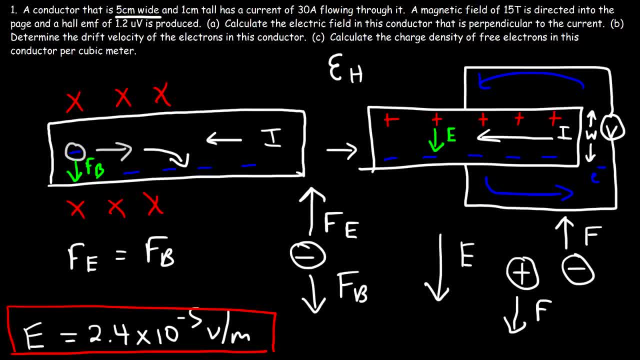 know that there's going to be a build-up of negative charge and there's going to be a build-up of positive charge. Now, this doesn't continue forever. The magnetic force is fixed as the electrons are moving towards the right, And so the electric field increases as the charge separation increases. Eventually, the 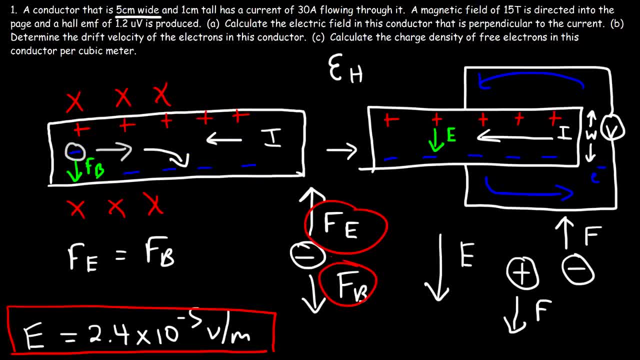 electric field gets strong enough where these two forces are equal. At that point the electrons no longer begin to drift towards the bottom. Instead, they're just going to keep flowing in this direction. They will reach a state of equilibrium. The magnetic force wants to bring them down, but these electrons are attracted. 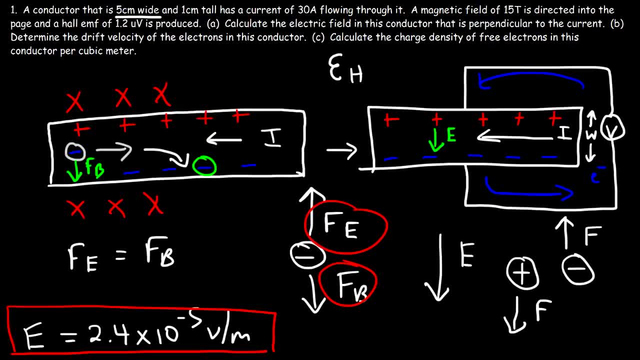 to the positive charge on the other side, And so when those two forces balance out, then the electrons will just travel to the right, and then we're going to have a steady-state voltage across the conductor. So now that we set the electric force and the magnetic force equal to each, 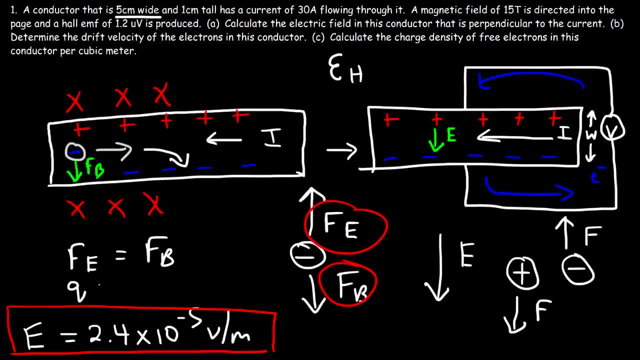 other. we can replace the electric force with the charge times. the electric field And the magnetic force is bqv. the magnetic field times, the charge times, the drift velocity. Now we could divide both sides by q, And so the drift velocity is equal to the electric field divided by the magnetic field. 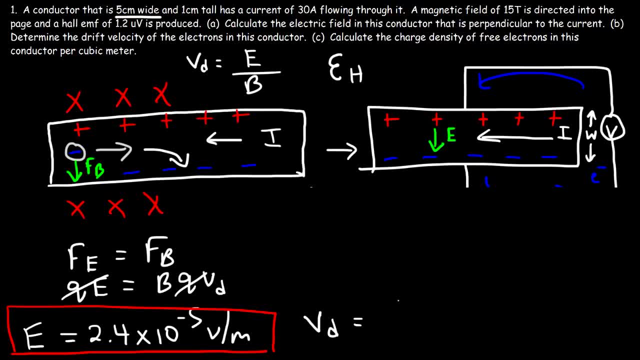 So the drift velocity is going to be 2.4 times 10 to the minus 5 volts per meter divided by the magnetic field of 15 Tesla, And so that's going to be 1.6 times 10 to the negative 6 meters per second. 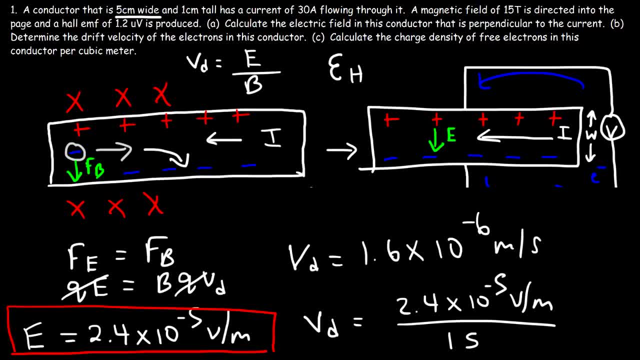 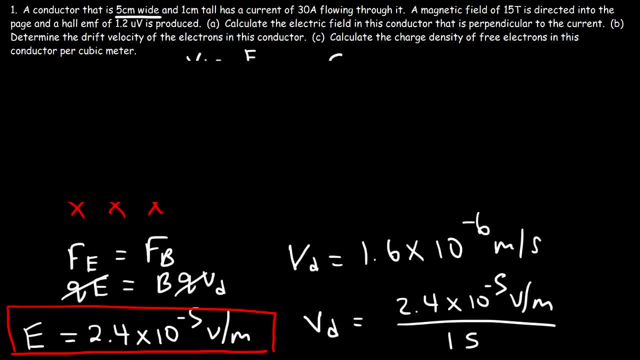 So now let's calculate the charge distribution. We're going to have the charge density of free electrons in this conductor per cubic meter. The current is equal to nqvd times a. N is the charge density, It's the number of free electrons per cubic meter in the conductor. So looking for n in this: 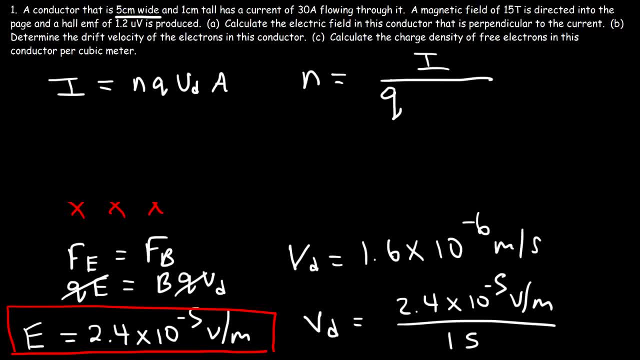 example. So it's the current Times, the charge of an electron times, the drift speed times, the cross-sectional area through which the current flows through. So let's talk about the cross-sectional area for a second. So let's draw a picture, basically the side view of the conductor. 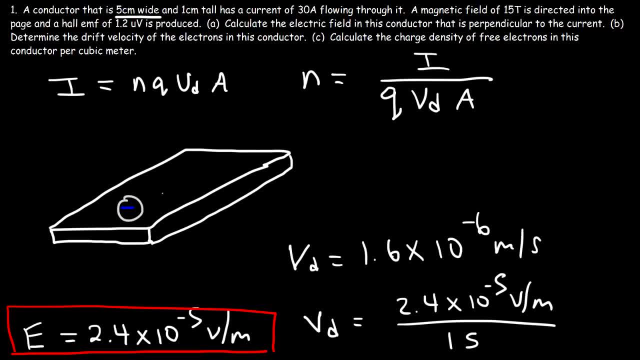 So here's the electron. It wants to move in this direction, but the magnetic field will cause it to move in this direction, And so this side will have a buildup of negative charge and this side will have a buildup of positive charge. So L. 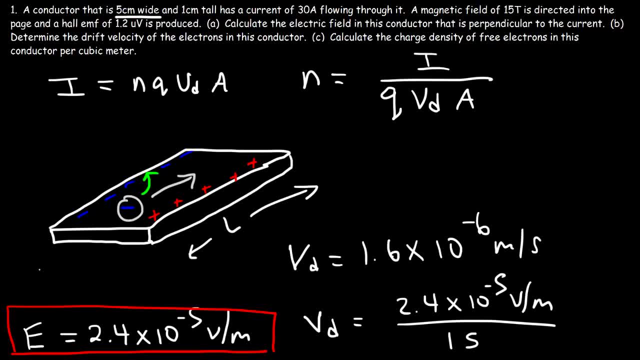 represents the length of the conductor, W represents the width, That's the distance between the negative charges and the positive charges, And D will represent the thickness of the conductor. So the cross-sectional area through which the current flows is this section highlighted in blue. So it's the width. 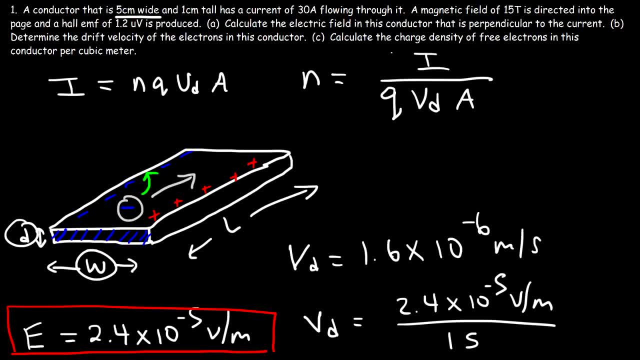 times the thickness D. So now we can calculate n. So it's going to equal the current, which is 30 amps, divided by the charge on an electron. We don't have to worry about the negative sign. And then the drift speed is 1.6 times 10 to the minus 6.. And then the 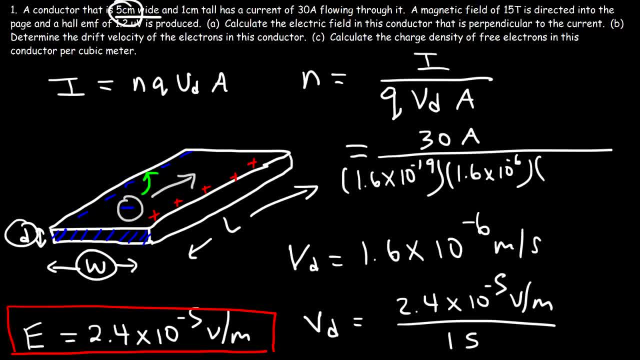 cross-sectional area. we have the width times the thickness, So 5 centimeters is 0.05 meters and 1 centimeter is 0.01 meters. So let's go ahead and find out what this is going to be. 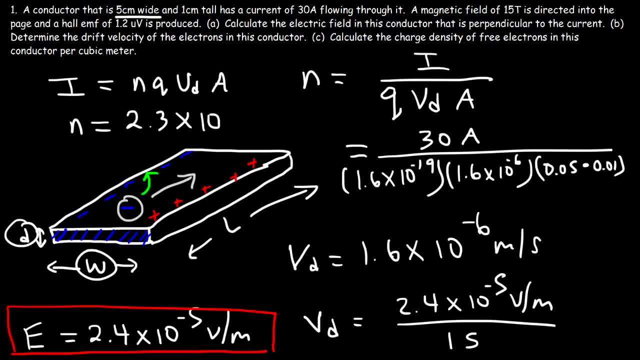 So n in this example is 2.3 times 10 to the 29 electrons per cubic meter. So that's the charge density of free electrons in this conductor. Now there's another formula in which you can get the same answer, And it looks like this: 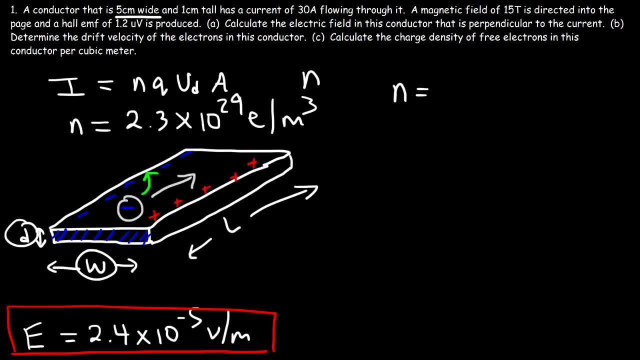 Perhaps you've seen this formula. So n is equal to the current density times the magnetic field divided by the charge times the electric field. Now the current density J is the current divided by the area, And so the current is 30 amps and 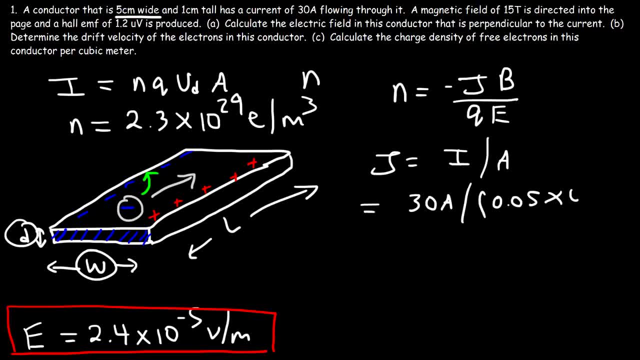 the cross-sectional area is 0.05 times 0.01.. And so the current density is 6 times 10 to the 4 amps per square meter. Or you could say 60,000 times just 60,000 amps per square meter. So n is going. 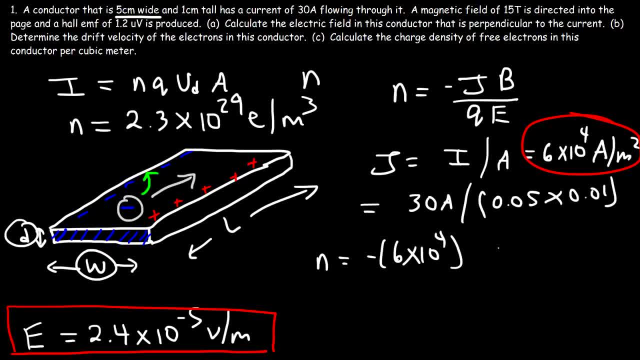 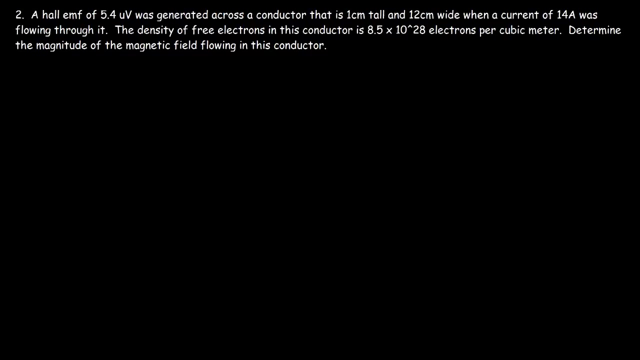 to equal J times the magnetic field of 15 tesla, divided by the charge times the electric field. So this time we'll have to use a negative sign And this will give the same answer of 2.3 times 10 to the 29 electrons per cubic meter. 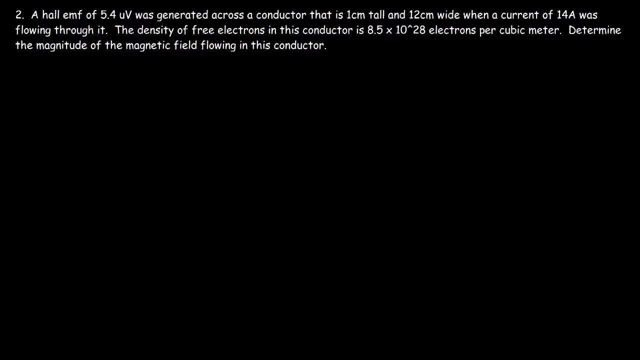 A Hall EMF of 5.4 microvolts was generated across a conductor that is 1 centimeter tall and 12 centimeters wide, when a current of 14 amps was flowing through it. Now we're given the density of free electrons per cubic meter. 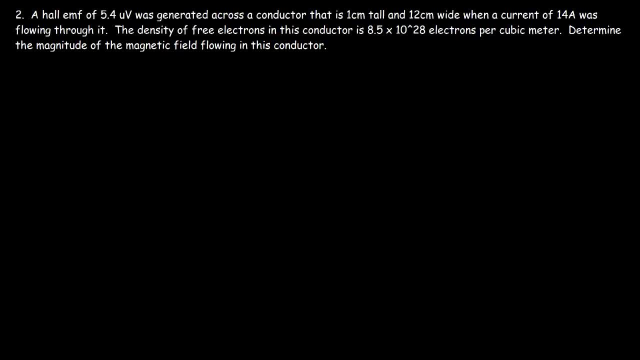 Determine the magnitude of the magnetic field flowing in this conductor. So let's draw a picture like the one we had last time And let's say we have an electron that wants to go in this general direction And we're going to have a magnetic field that comes, let's say, out of the page. 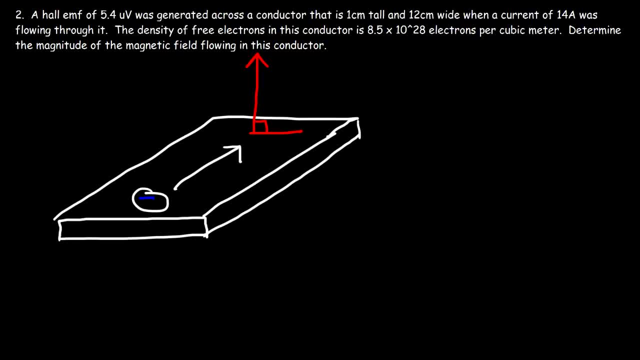 So, using the right hand rule, where is the electron going to go? So, if you point your four fingers out of the page and your thumb in the direction of the current, a proton will feel a force that comes out of the palm of your hand, which is to 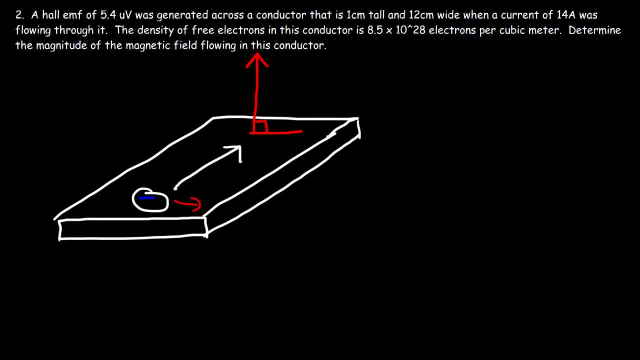 the right, So a proton will accelerate in this direction, but the electron will accelerate in this direction. So we're going to have a buildup of negative charge on the left side and a buildup of positive charge on the right side, And so we could connect a voltmeter across. 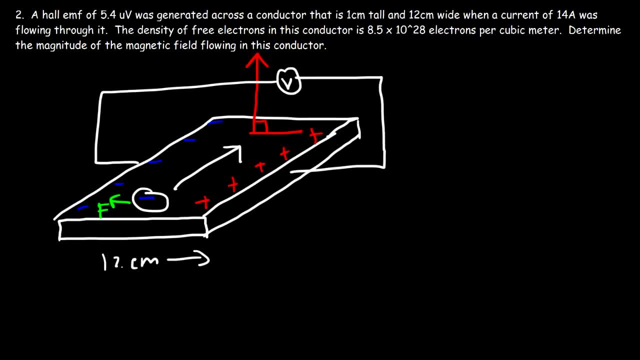 Now we have the width of the conductor is 12 centimeters wide And we have the thickness: It's one centimeter tall. So how can we calculate the magnitude of the magnetic field passing through this surface? Well, we know that the drift speed is equal to the electric field divided by the magnetic 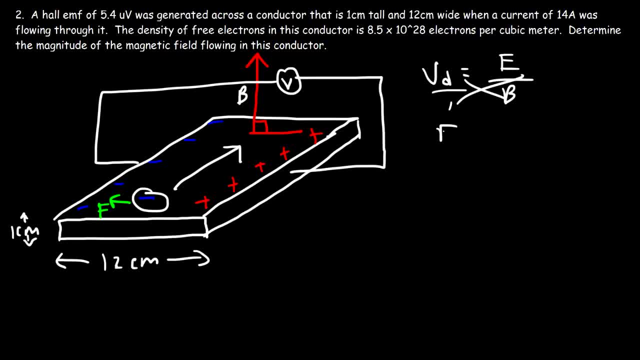 field. So if we cross multiply E is going to equal B times VD. Okay, So the magnetic field is equal to the electric field divided by the drift speed. The electric field is equal to the Hall EMF divided by the distance between the positive 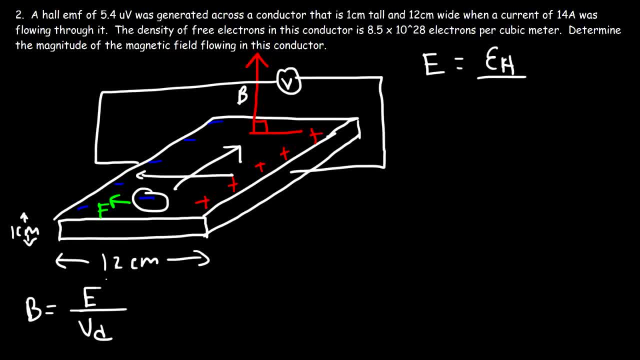 and the negative charges, which is W, And so we can replace E with that. Now to calculate the drift speed, we can use this equation. So the drift speed is going to be the current divided by NQ times A. So B is equal to E times 1 over VD. 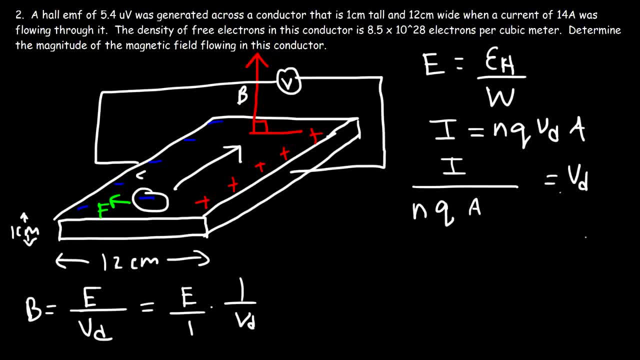 And if we flip both sides, 1 over VD is NQ times VD, NQ times VD is NQA divided by the current. So we can replace E with this term. So it's the Hall EMF divided by the width. 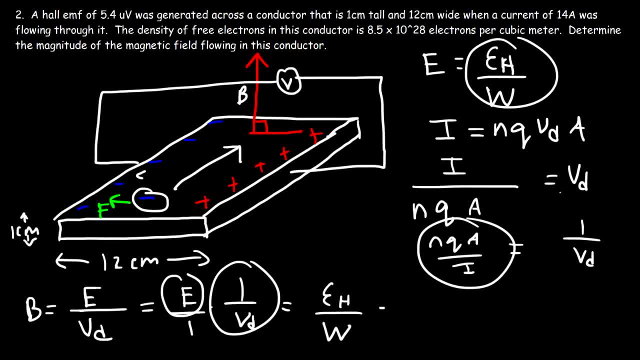 And then we can replace 1 over D with this term, So times NQA divided by the current, Now A, the area, as we said before, is the area of this region. So it's the width times the distance. Okay. 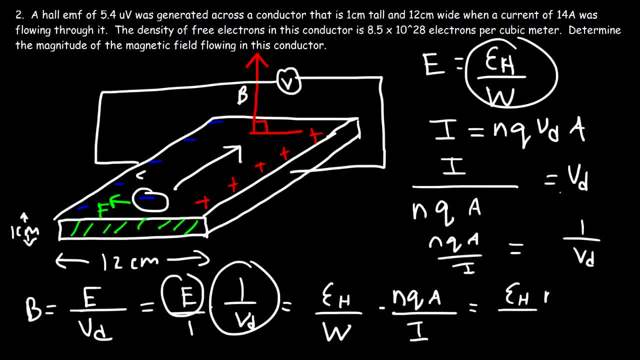 The thickness, so W times D. So therefore we could cancel these two terms And this will give us a general formula for the magnetic field. So the Hall effect can be used to measure the magnetic field passing through it by measuring the EMF produced, if you know the current flowing through this conductor. 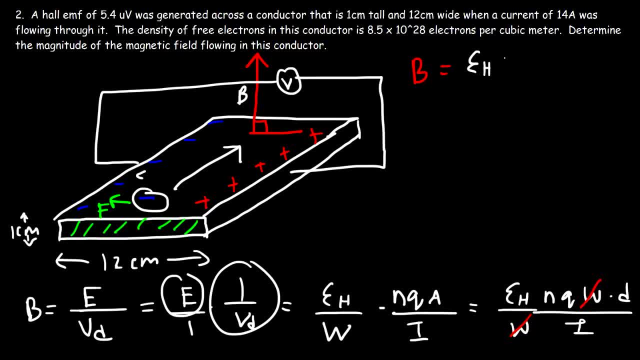 So the magnetic field depends on The EMF measured times the charged density of free electrons in the conductor times the charge of an electron, which is a fixed value, times D, that is the thickness of this part of the conductor divided by the current. Now let's go ahead and finish this problem. 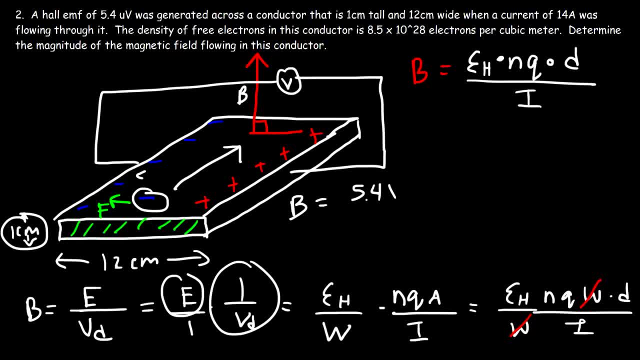 So the Hall EMF is 5.4 microvolts, or 5.4 times 10 to the minus 6 volts. N is 8.5 times 10 to the 28, and the charge is 1.6 times 10 to the negative 19.. 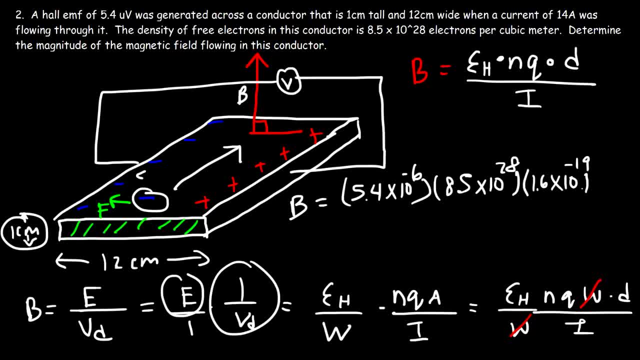 And then D. let's see. the thickness is 1 centimeter, so that's 0.01 meters divided by the current, which is 14 amps in this example. So let's see what this is going to come out to be. 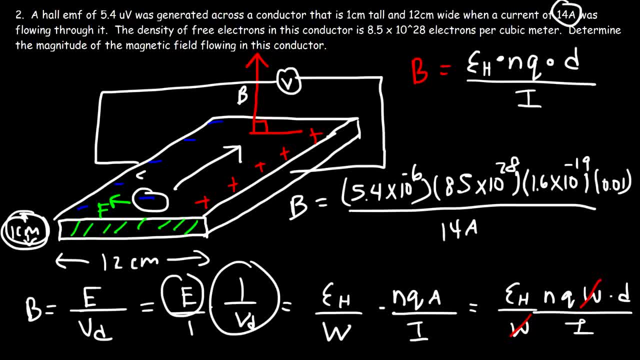 So what I have is 52.5 Tesla. So that's the strength of the magnetic field in this example. So now you know how to use the Hall effect to measure the magnetic field that passes through the conductor. So you have to measure the voltage and you can determine the thickness, because that's 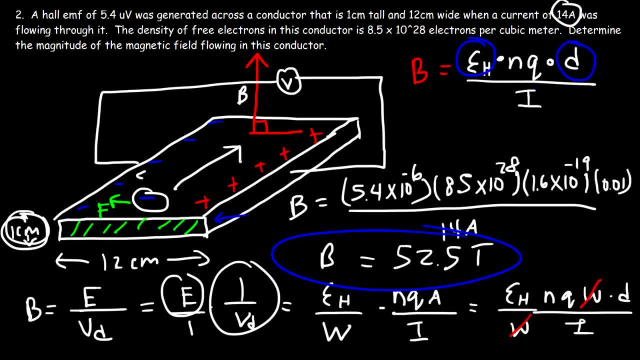 just based on the conductor. You can measure that And you need to measure the current that's flowing through it. So by keeping the constant current flowing through the circuit and knowing the thickness of the conductor and at the same time you need to know the number of free electrons.